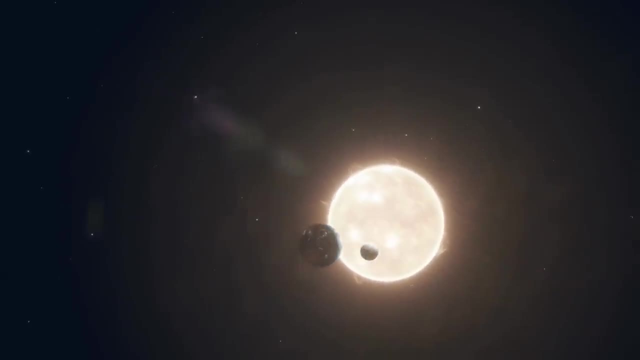 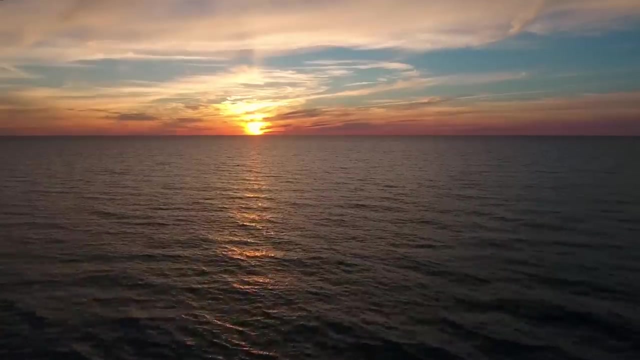 habitable zone. Now in the solar system there are three planets in the habitable zone. there's Venus, Mars and Earth. Venus is close to the sun, Mars further away, All of those planets that we think had water on the surface, So they all could have been habitable in that sense. And 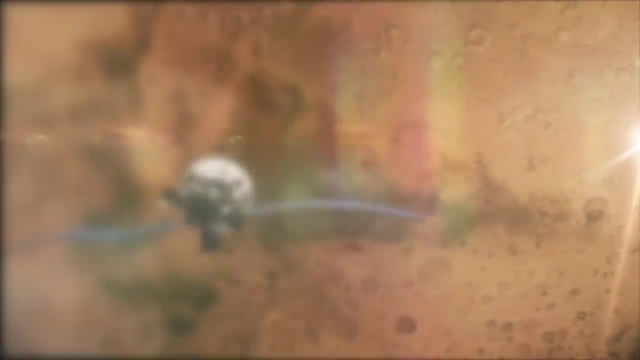 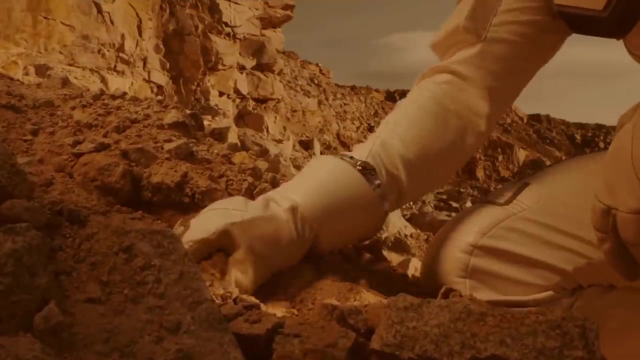 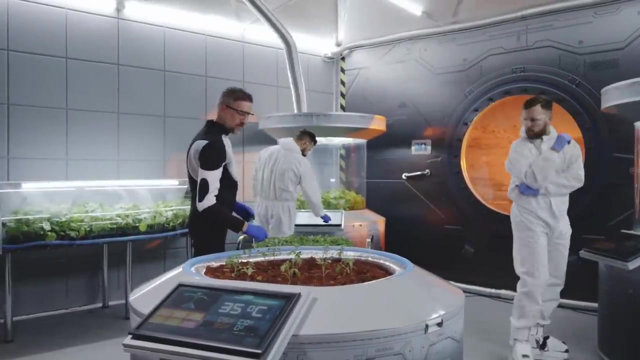 still. you know we're looking for life on Mars to this day. Of course, finding life on Mars would be undoubtedly among the biggest discoveries in human history, But if there is life on Mars, most scientists think it's microbial life, The more interesting kind of life we hope to discover. 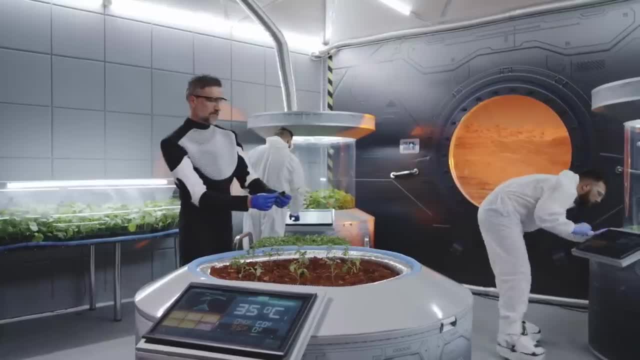 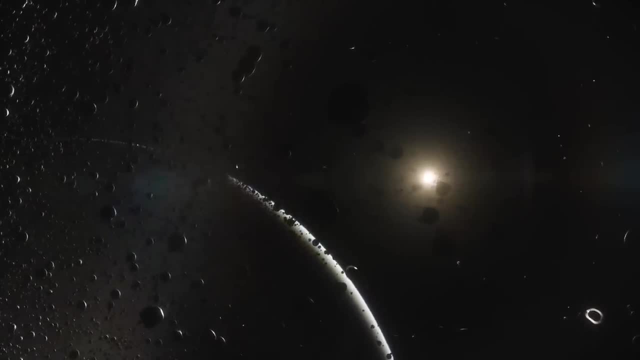 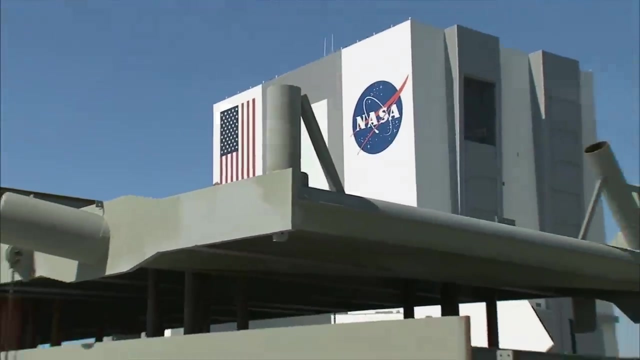 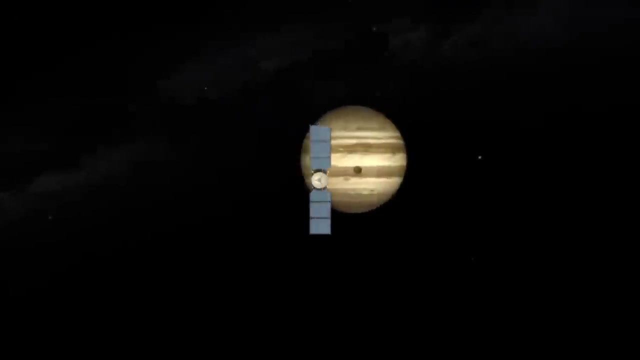 that would change our worldview forever is multicellular life, such as plants or animals. Luckily for us, there is a place within our solar system that might host that kind of life: Enter Jupiter's moon, Europa. NASA is preparing the Europa Clipper mission, which would launch in October 2024 and will arrive in 2030.. The mission is 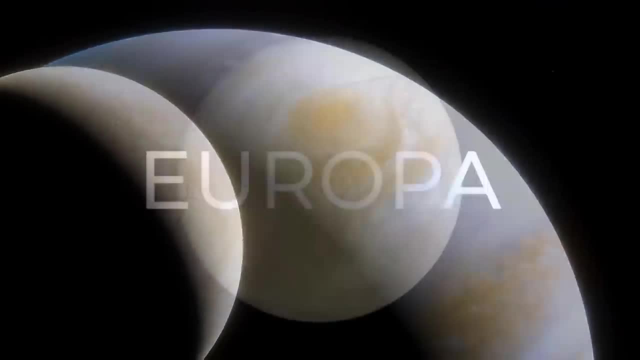 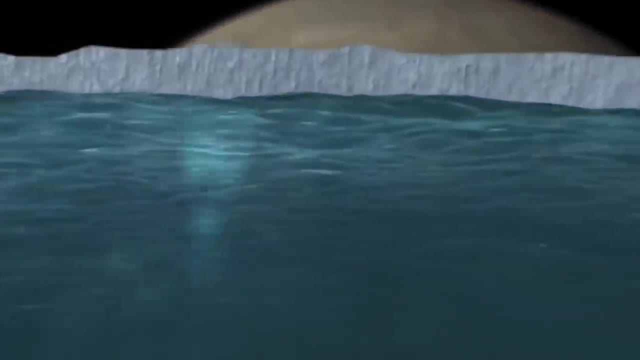 currently planned to conduct four years of science observations at Europa. This moon shows strong evidence of an ocean of life. It's a very strong evidence of an ocean of life. It's a very strong evidence of liquid water beneath its icy crust. So it's a top candidate to explore and hopefully, 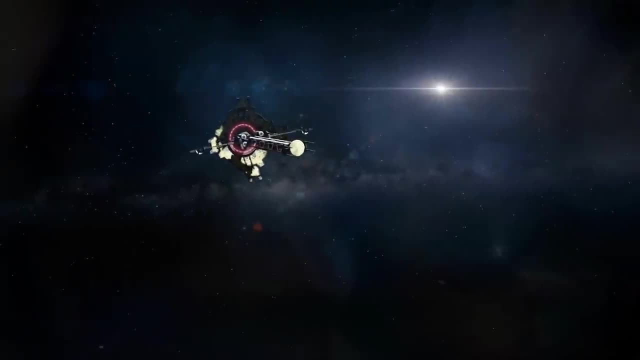 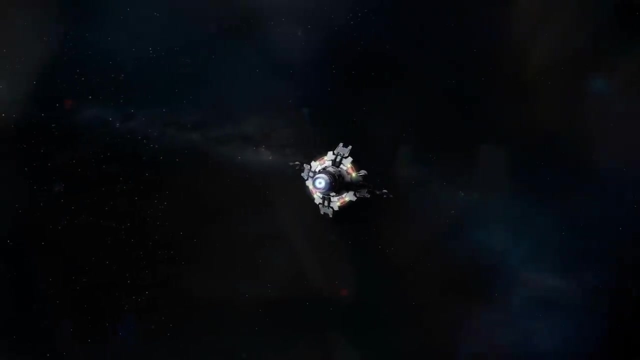 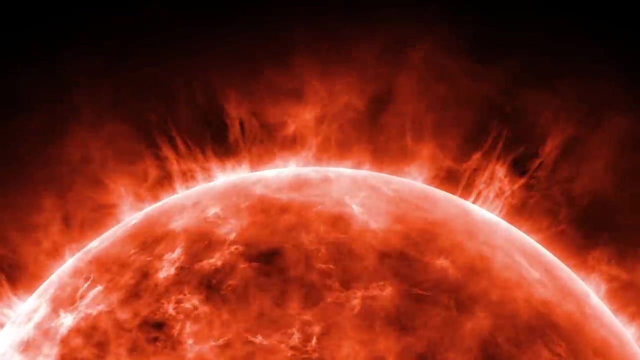 we will find evidence of alien life Going beyond our solar system. it's extremely difficult, if not impossible, with our current technology to send space probes and find evidence of alien life. As the nearest star to our sun, Proxima Centauri, is about 4.2 light years away. 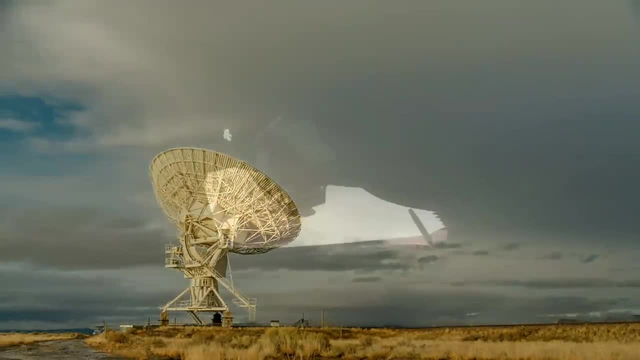 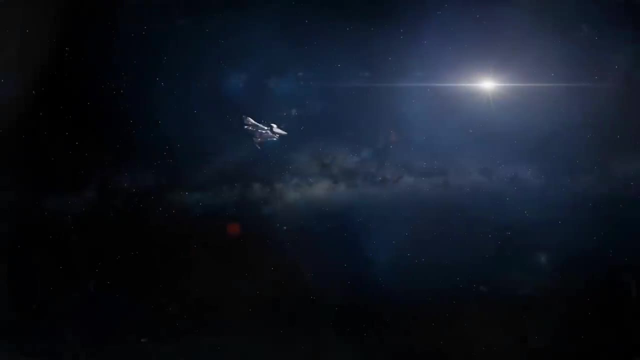 So the best method is to stay put and listen for radio signals or direct our telescopes At the location of exoplanets and look out for biosignatures. Obviously, the most exciting type of hierarchy of alien life is intelligence. It is estimated that with our current pace of 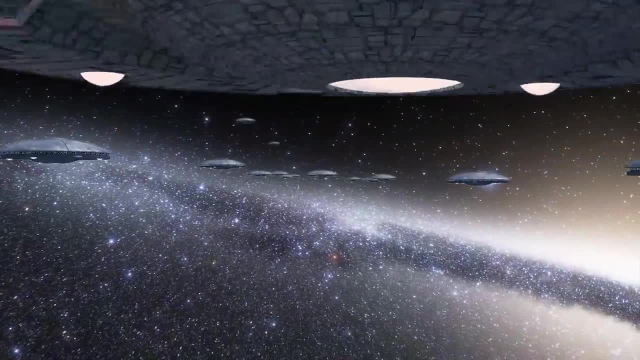 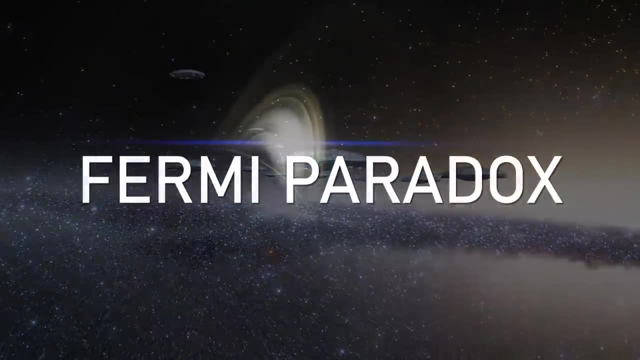 technological growth, a civilization can colonize our whole galaxy within 10 million years. And if that is the case, where is everybody? The flip side of this is there are loads of planets out there And there's been loads of time. This has got a name. actually It's called the Fermi. 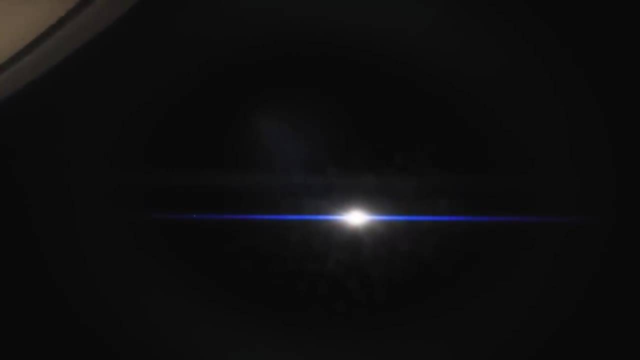 Paradox after someone called it Fermi, And it's called the Fermi Paradox after someone called it Fermi. It's called Enrico Fermi, a great Italian physicist who asked this very simple question, which is: where are they? Because, given the number of planets, given the number of stars, 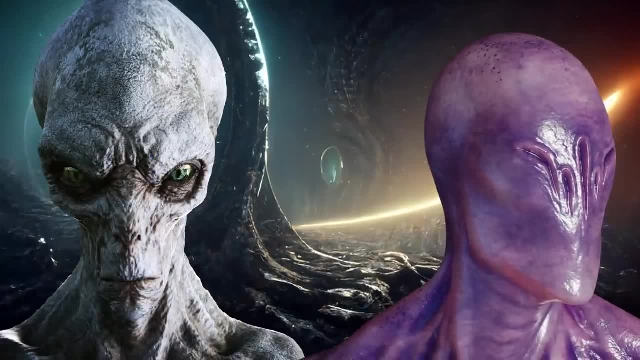 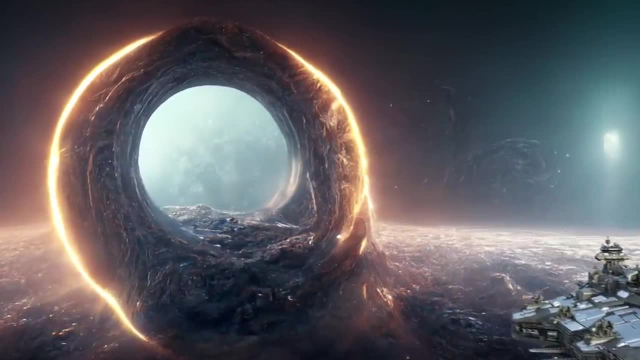 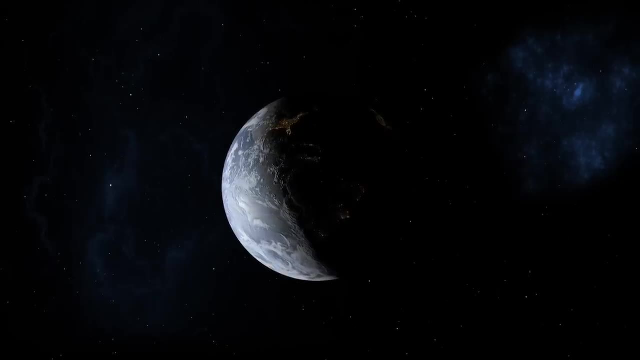 and given the amount of time in this galaxy for complex life to emerge, it seems as if at least a few civilizations should have become a space-faring civilization. So part of the evidence, part of the great conundrum here, is that so on the one side, yes, we've got the history of life. on Earth, which says that we took a long time to emerge. But on the other side, we've got the history of life on earth, which says that we took a long time to emerge. But on the other side, we've got the. 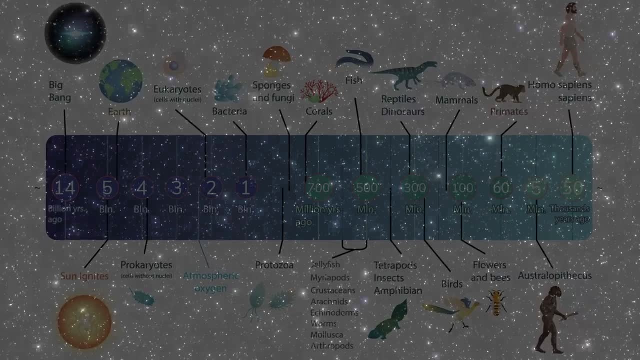 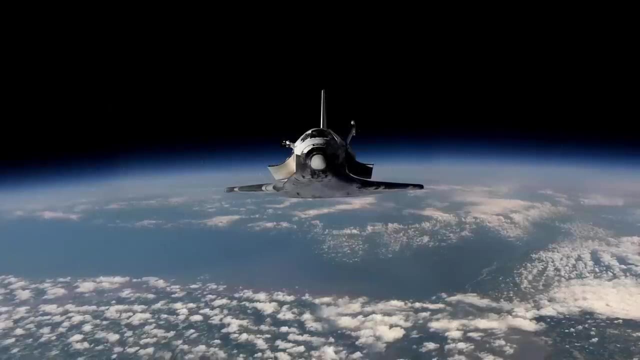 history of life on Earth, which says that we took a long time to emerge, And so it looked quite like an unlikely process. On the other side, you've got all this real estate and you have this. if you think about where we could go, what could we become as a civilization So already? 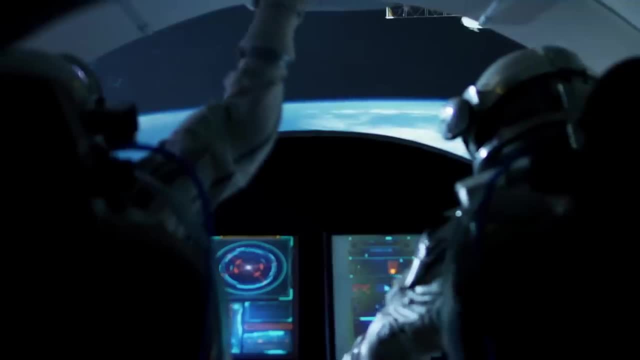 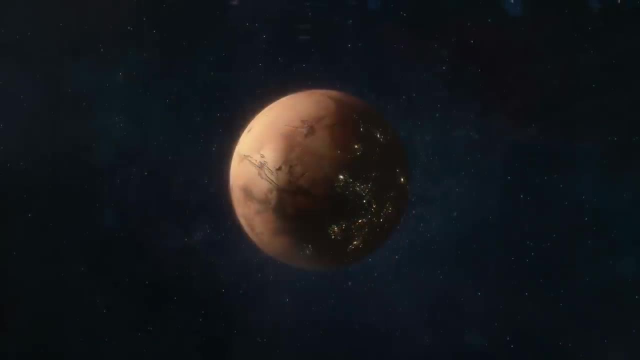 we are becoming a space-faring civilization now very quickly. So give us 1000 years. we don't destroy ourselves or do anything stupid. We're, I'm sure, we're going to be on Mars, we're going to be on the moon. we're going to be thinking, perhaps. 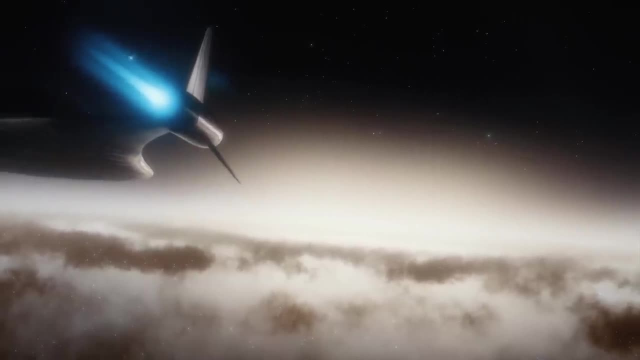 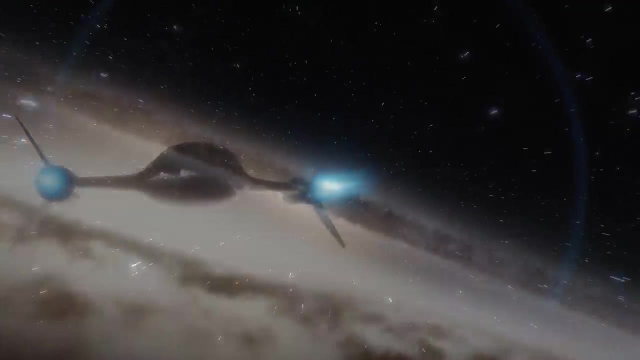 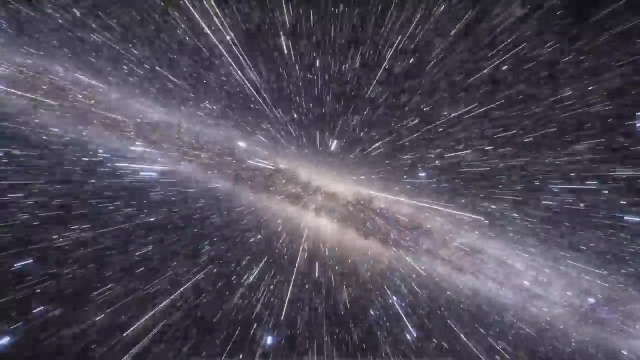 taking our first steps out to the stars. give us a million years, one million from now. if we survive, we should become a space-faring civilization. now, one million years. the galaxy has been around for the age of the universe- 12, 13 billion years. so it only takes a few civilizations to have evolved a 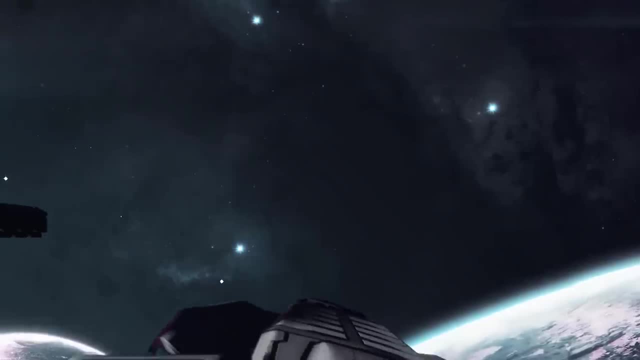 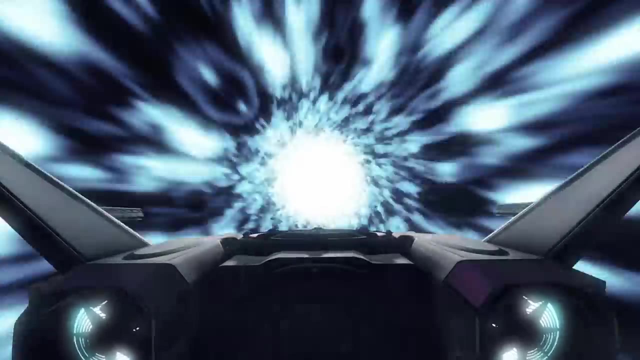 bit ahead of us. a million years, let's say a billion years. a billion years, it's still nothing. you get some civilizations that evolved a billion years before us. why can't we see them? so then people start saying, well, maybe there's a finite life that all civilizations have. maybe they. 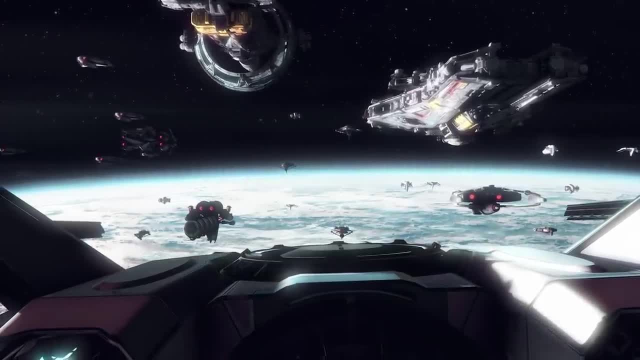 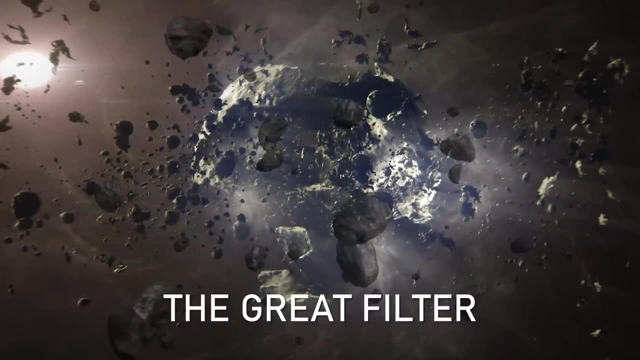 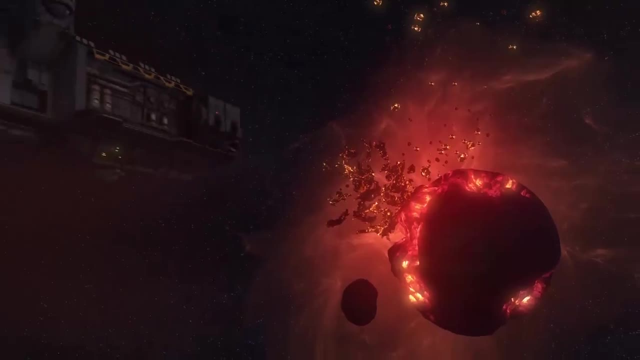 destroy themselves. maybe they don't become space-faring civilization. one possible resolution of the fermi paradox is the great filter. it presupposes that in the development of life, from the earliest stages of abiogenesis to reaching the highest levels of development on the kardashev scale, there exists some. 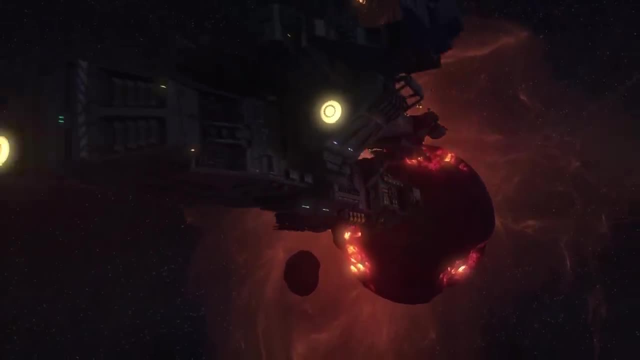 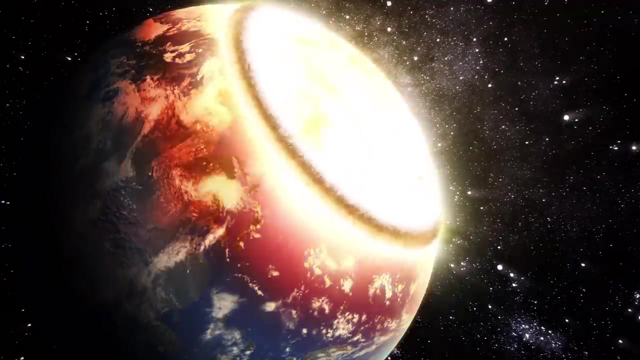 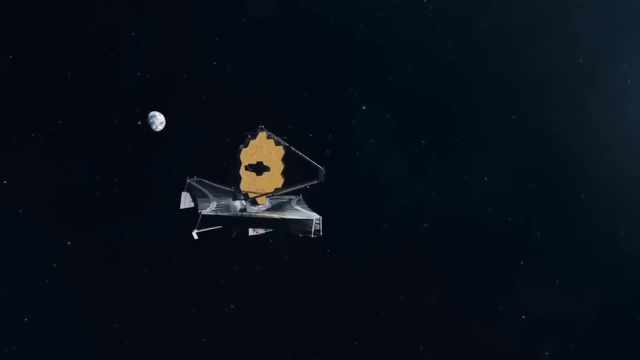 particular barrier to development that makes detectable extraterrestrial life exceedingly rare. this barrier to the evolution of intelligent life could be as a result of self-destruction. meanwhile, the evolution of telescopes that can detect techno signatures could provide insights into the great filter. if planets with techno signatures are abundant, then this can increase. 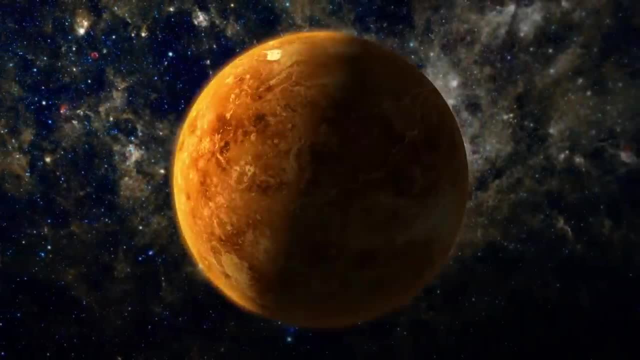 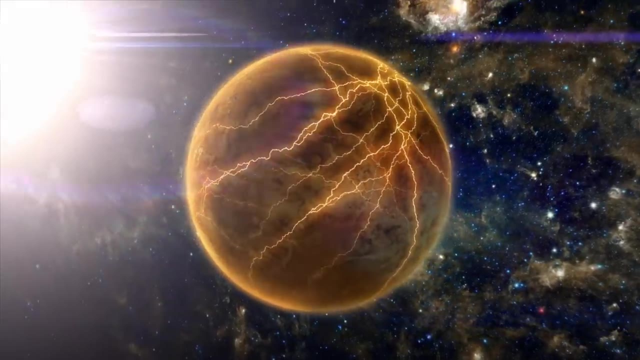 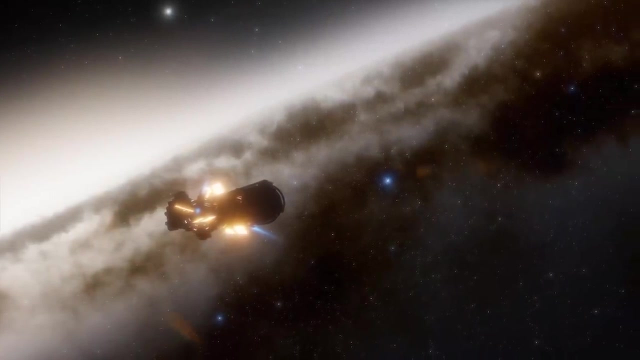 confidence that the great filter is in the past. on the other hand, if finding that life is common place with techno signatures are absent, then this would increase the likelihood that the great filter lies in the future. there is another relatively recent and quite interesting hypothesis that attempts to resolve the fermi paradox: if an extraterrestrial species becomes advanced, 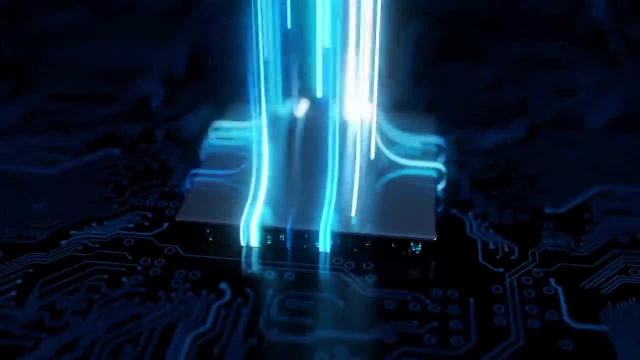 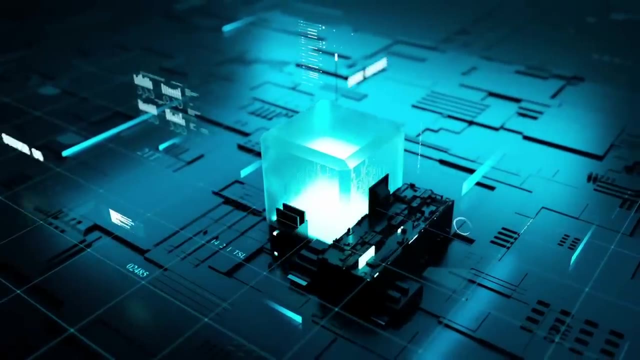 enough to send signals we can pick up. it will likely shed its traditional biological form and become a type of machine intelligent. within this hypothesis, it is speculated that a full digital civilization will be able to detect a large number of extraterrestrial life-forms in the future. 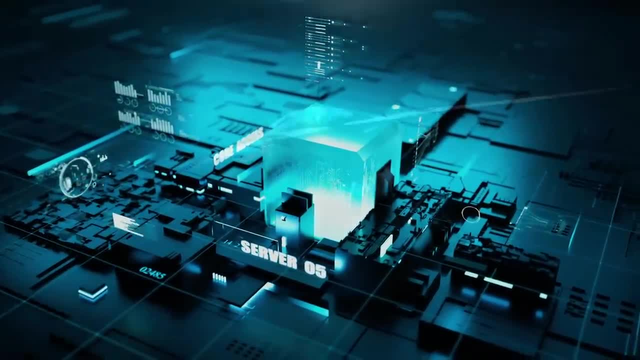 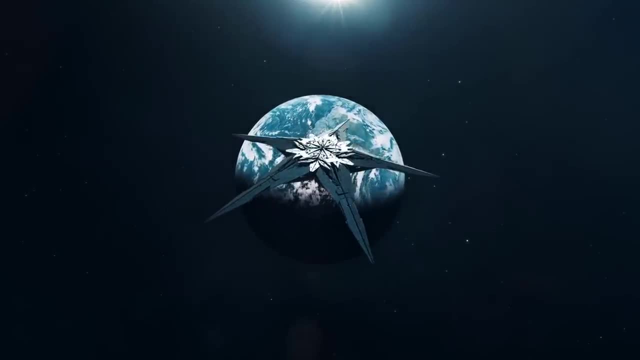 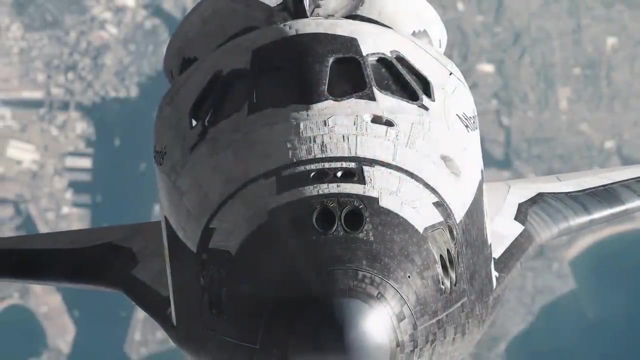 the other interesting solution to the fermi problem, which is popular among ufo fans, is the so-called zoo hypothesis, which entails we are being observed without our knowledge. there is also the depressing solution to the fermi paradox, which is that we're the first ones and will be extent long before any. 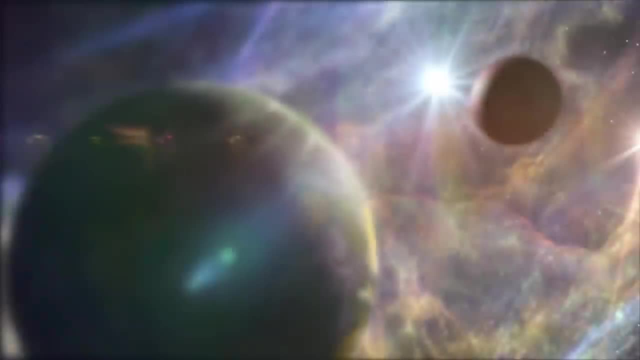 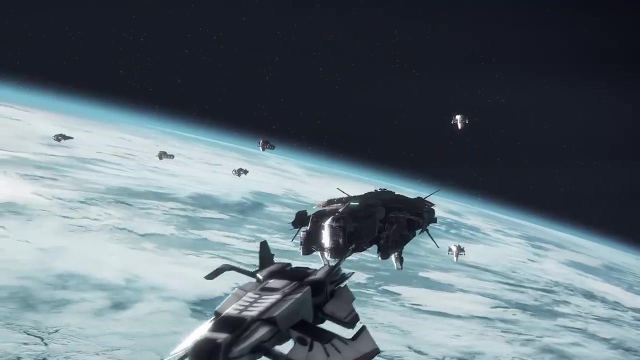 other civilizations emerge in our galaxy. what's interesting is, when you talk to astronomers, They say that we estimate there are 20 billion potentially Earth-like planets out there in our galaxy. Surely there must be life all over the place, Right? it's a guess, because we haven't. 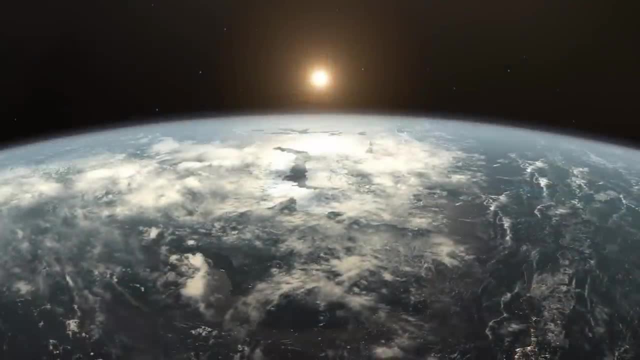 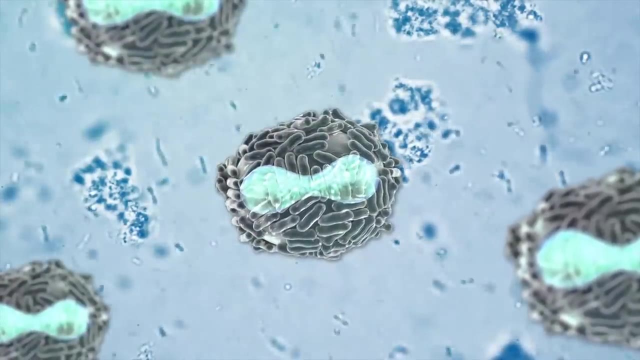 found any anywhere. But what we know from the history of life on Earth is that life began pretty much as soon as it could here on Earth. So we have good evidence that life was around, let's say, 3.8 billion years ago, So pretty much as soon as the Earth had formed and the oceans formed on the 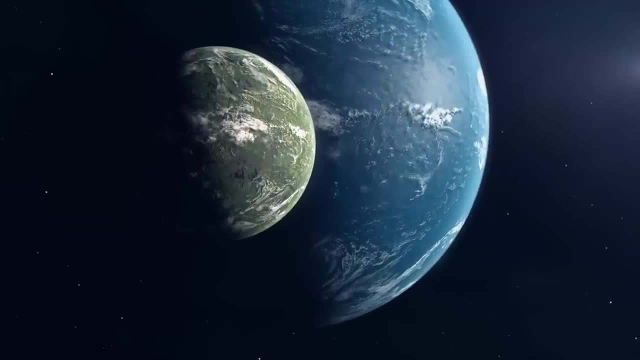 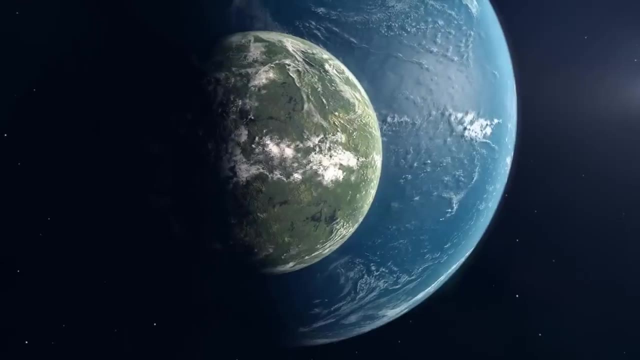 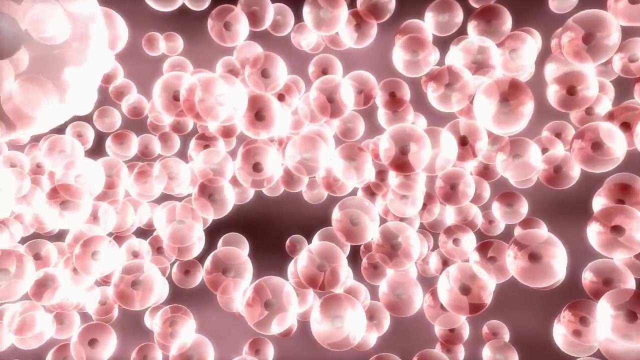 Earth you see evidence of life, So that might give you a sense that the origin of life on a planet might be a high probability, right given the right conditions, just because of what we see on Earth. But this is really important. Well, when did complex life appear? So not just single cells. 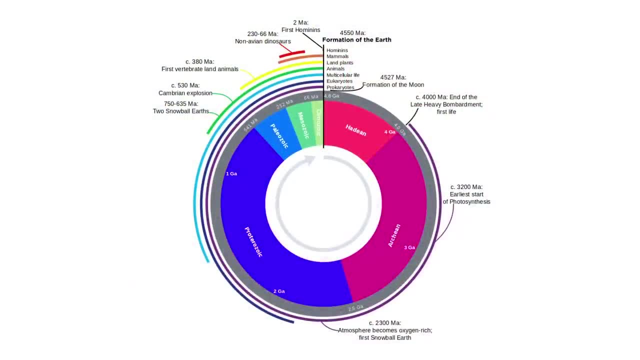 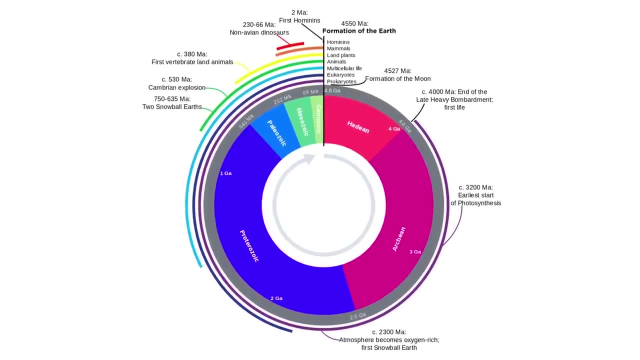 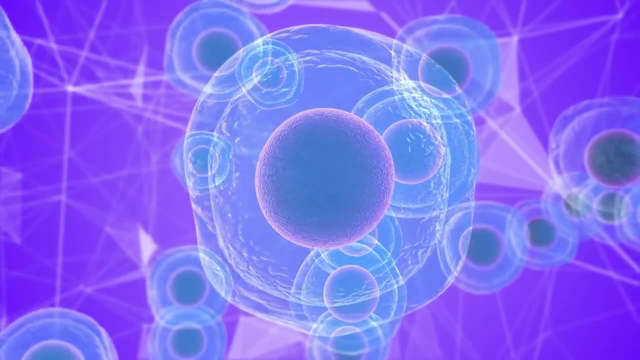 you know animals and plants. The evidence of complex multicellular things on Earth goes back, let's say, 600 million years, Not much further than that. So it's within the last billion. So on Earth what happened was that there were single cells, things doing interesting stuff, photosynthesis and things. But for let's